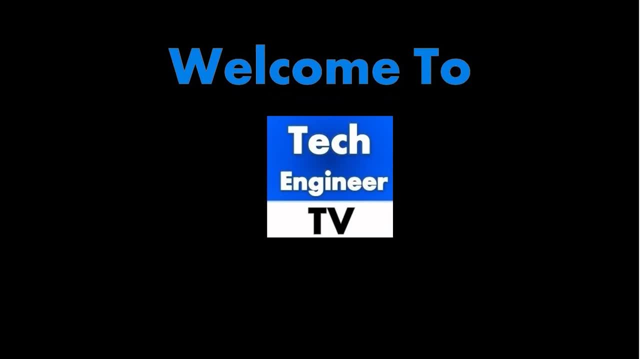 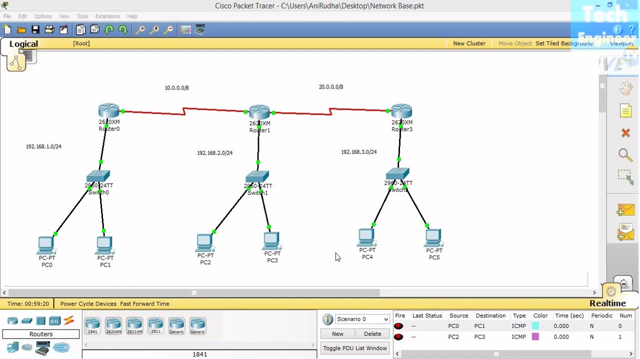 Hello there, In this tutorial I'm going to discuss about AD value, So administrative distance is known as for believability of router protocol, or you can say which routing protocol is most trusting one, because the most number of AD value means the less trusted protocol it is. So let me first show you the 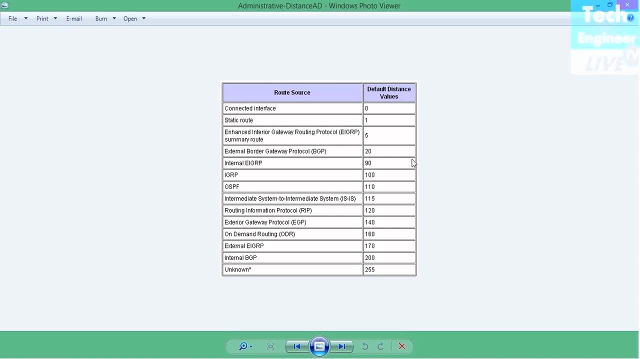 record. sir, This is the default distance value, the administrator distance value, AD value- and you can see the static route- is very less AD value have and internal BGP having a very big number of AD value means you can see EGP, for example, EGP or RIP. Their distance value, administrative distance value, is 120, 140. 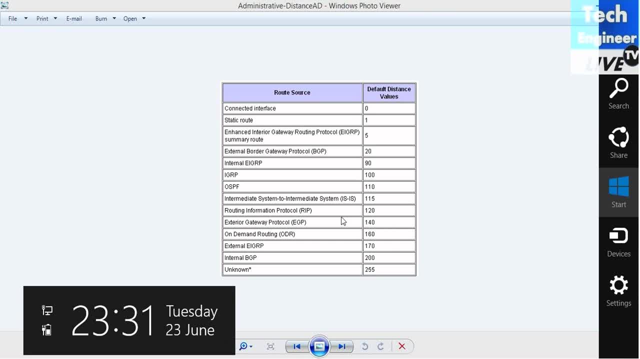 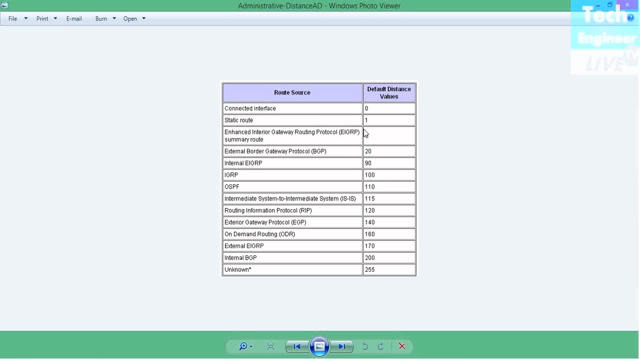 respectively. and the other value is, for example, static route. so they have one or EIGRP, five, ERGRP, summary route. having five, It means that static route is most trusted, most believable network and the EGP or RIP or external EIGRP or internal BGP are less trusted. This is the main. 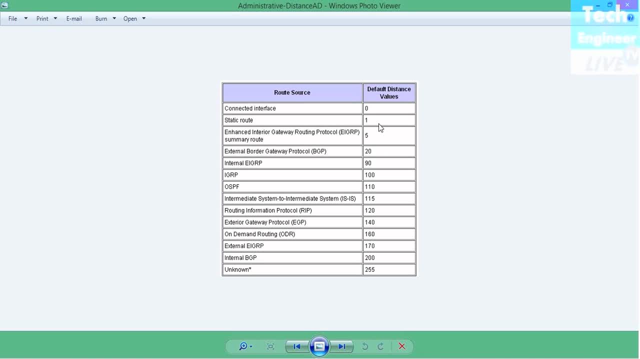 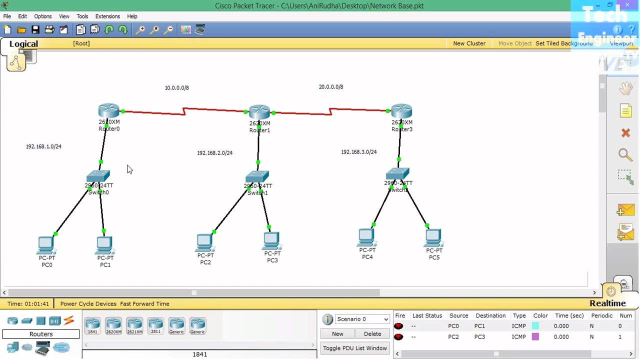 mode of AD value is that the less the value is, the more it believability and the more it trusting is. So this is where we're going to learn about in this tutorial about AD value. Let me open this chart Now. currently, our network is configured and 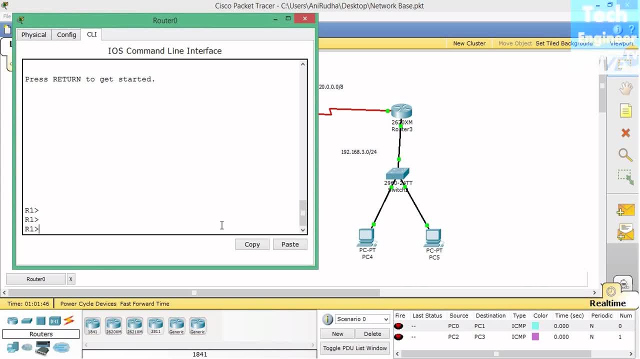 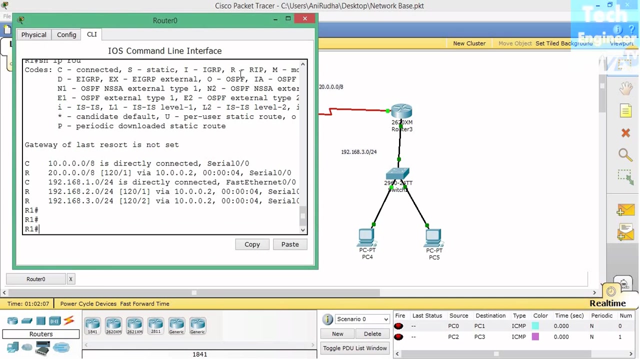 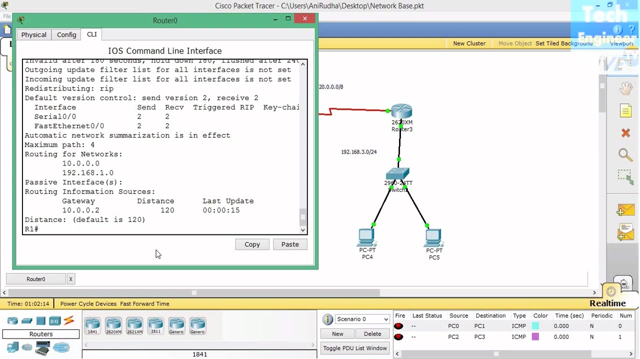 I'll show you enable Config terminal. or let me show: show IP route command. So currently it's routing is enabled via RIP. You can even go to show IP protocol. So currently our routing is enabled with RIP version 2.. So currently our routing is enabled with RIP version 2.. So currently our routing is enabled with RIP version 2.. 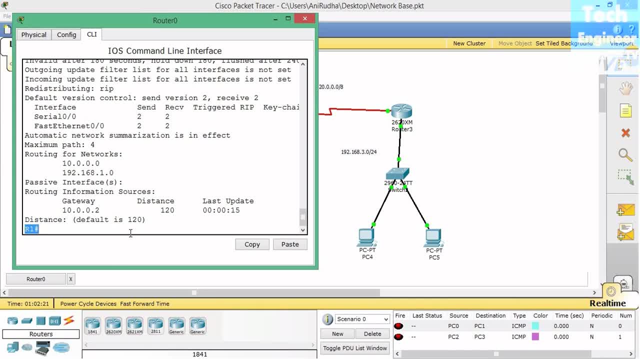 Now we work, we need to, and you can see the default distance value is 120.. RIP was split or anything else, to enable routing via ERGRP horizontal. we can see the default distance value is 120- 120. so when you wants to rings to a room once to enable routing via RIP version two. 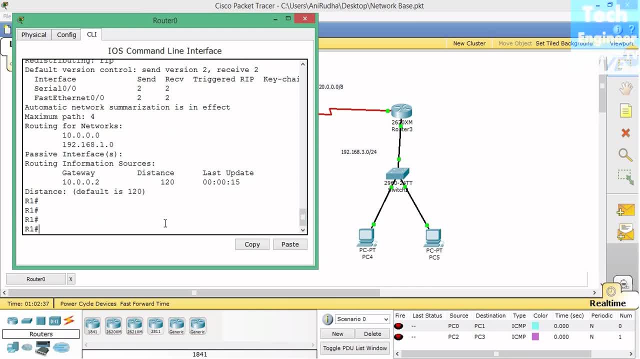 You can see the default distance value is 120. voeproxy, So for example, a config and router space RIP. Power Supply k, So for example, a config k ERP, for example some ES number, autonomous system numbers, for example, give a 20 and then network ID: 192, 192 dot, 168 dot, 0 dot. 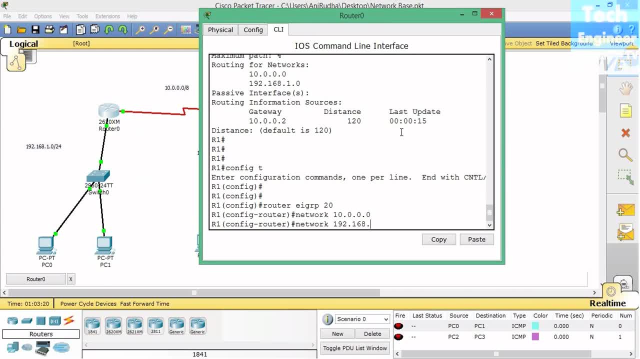 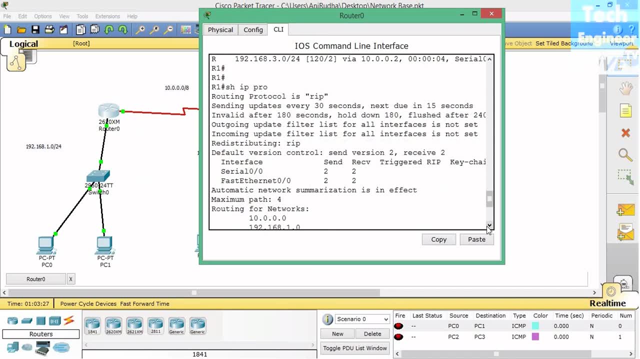 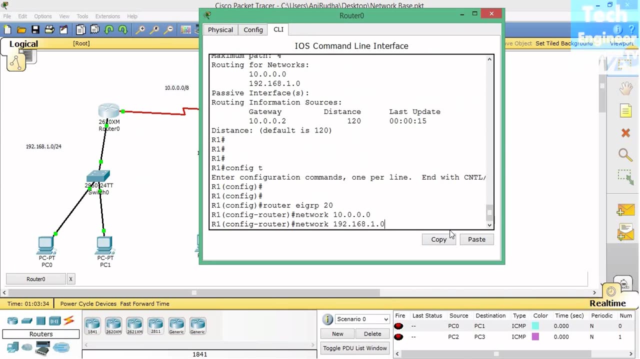 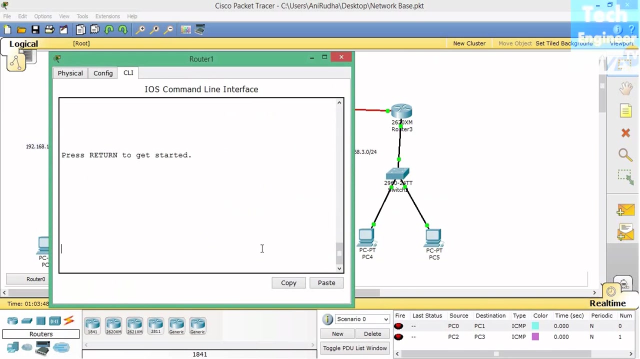 let me show you: okay, 1.0, 1.0. so it's done. now let me able same in this network also. it's a rip, but we have to first configure it: router EIG, the RP 20, 20 network, for example, pants 0. 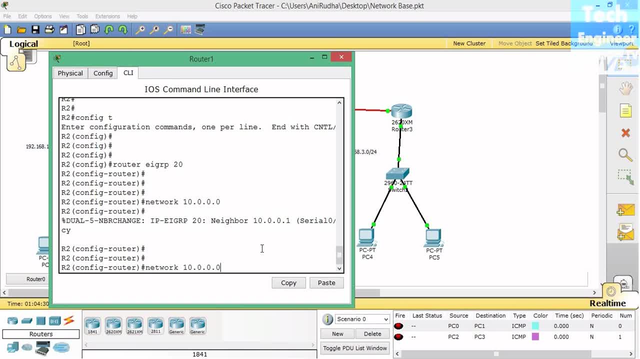 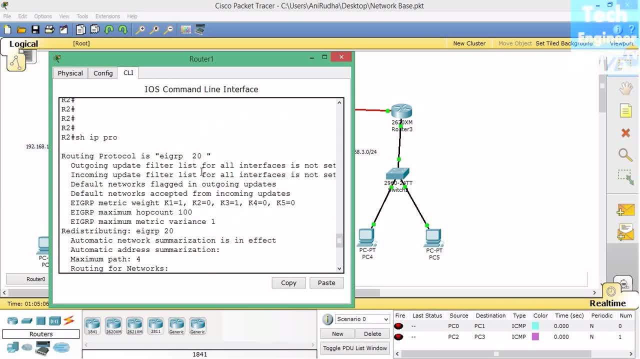 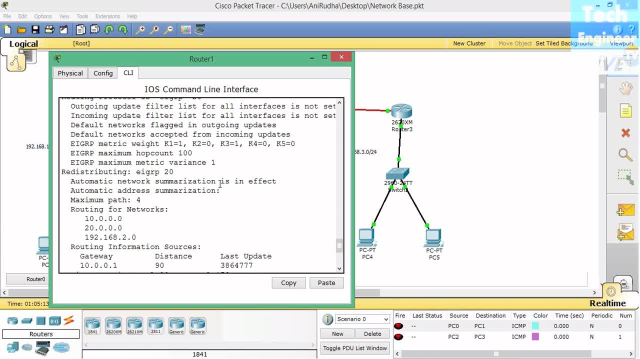 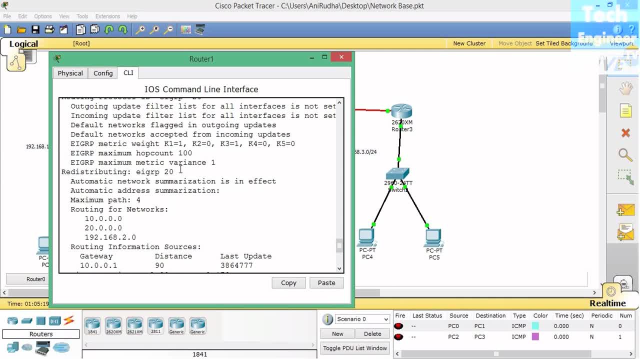 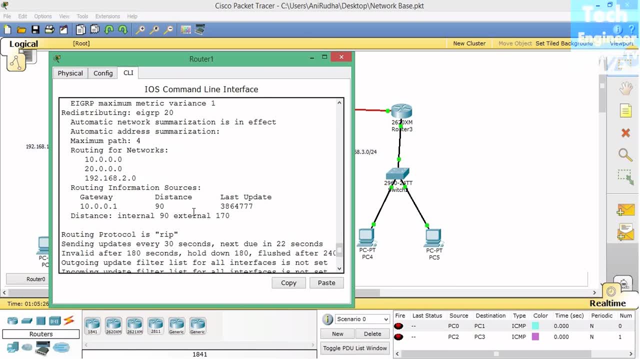 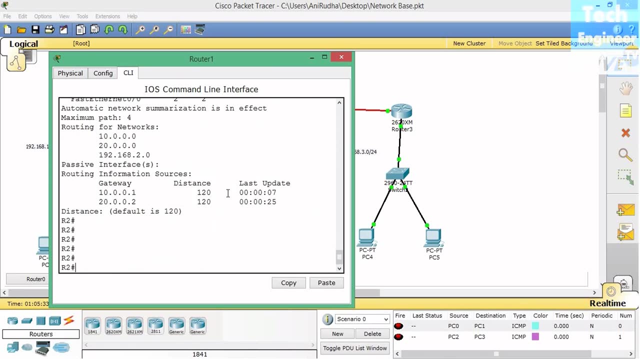 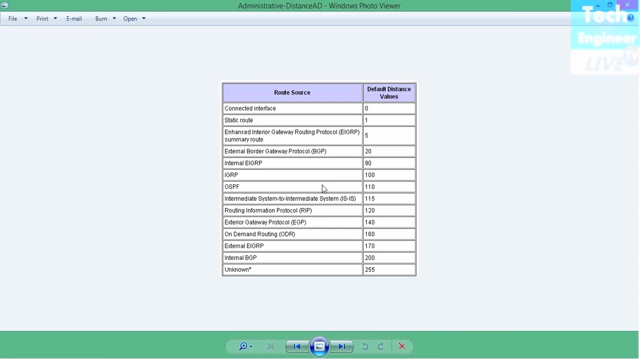 1.0, 1.0, 1.0, 1.0, 1.0. distributing all this thing at their distance is: internal distance is 90, external 170, distance is 120. so EIGRP will learn about that. have a 5 internal EIGRP. 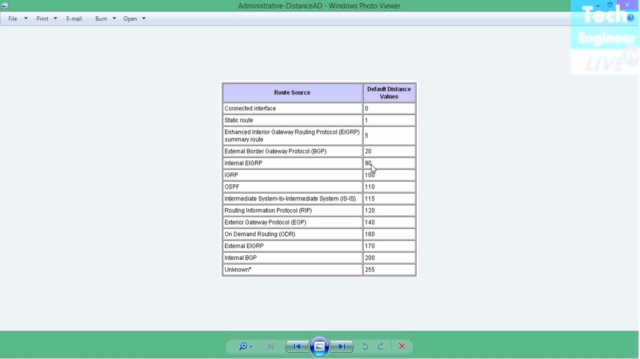 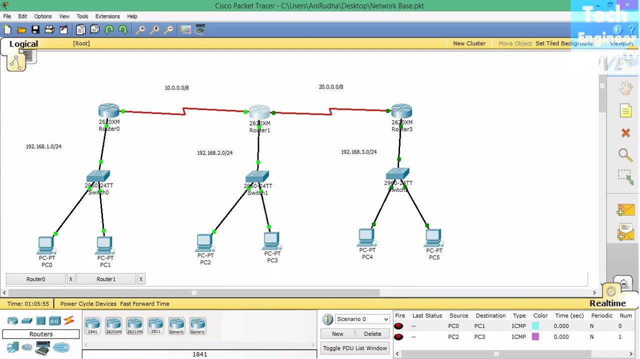 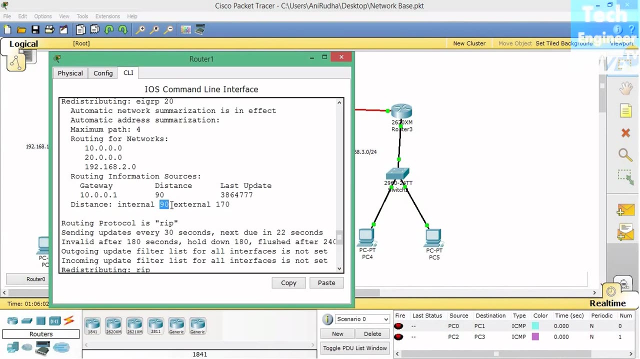 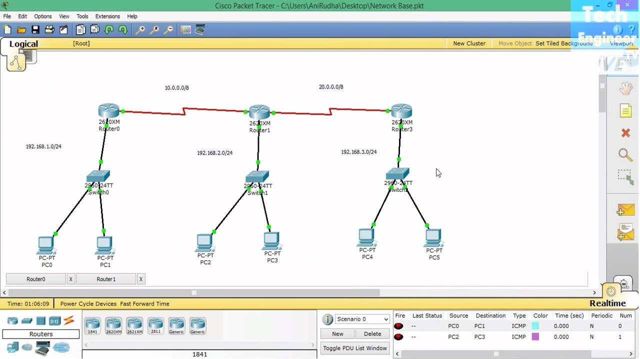 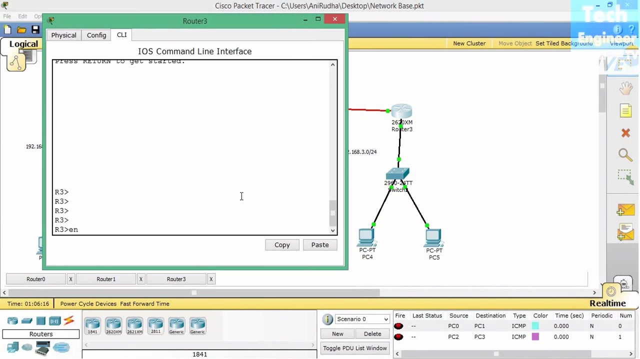 having 90, and this is where we are we are getting. let me show you this is where we are getting from router run here we'll have 90 internal EIGRP, so 90, okay, so enable EIGRP here. also. configure key now: router EIGRP 20 network. 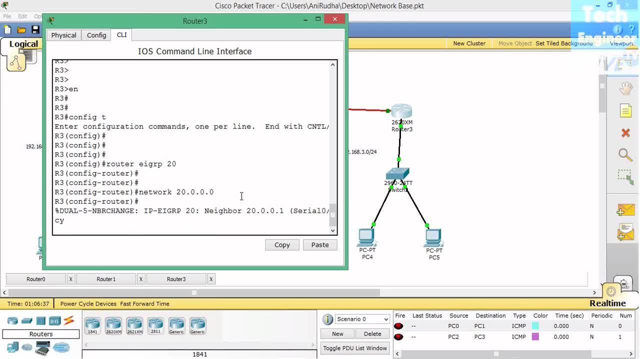 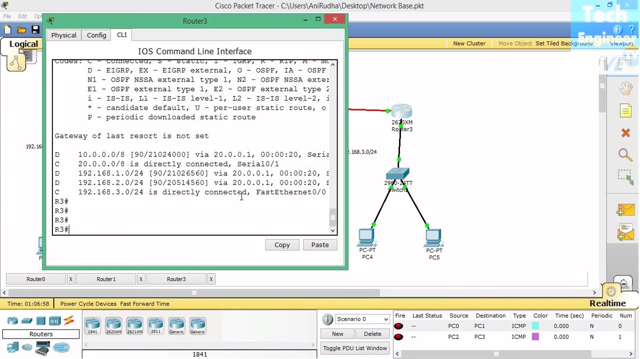 20: 0, routing is done. routing is done 192.168.3.0, so show IP route command or, for briefly, show ip protocol. not here, honey. now here me. have enabled the routing via a 90.168.3.0. っぱ FI absolute knife. 브�谷连다 нап". 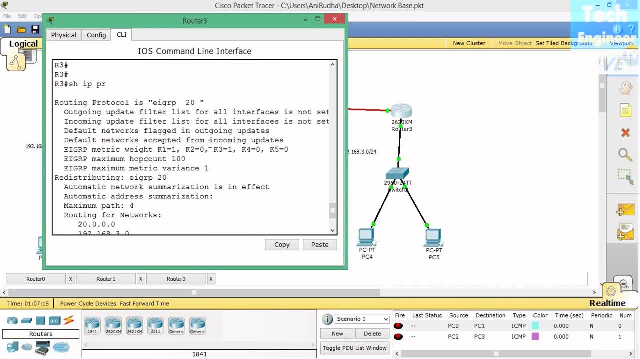 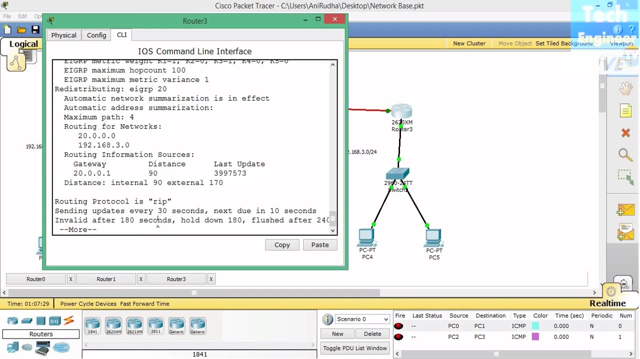 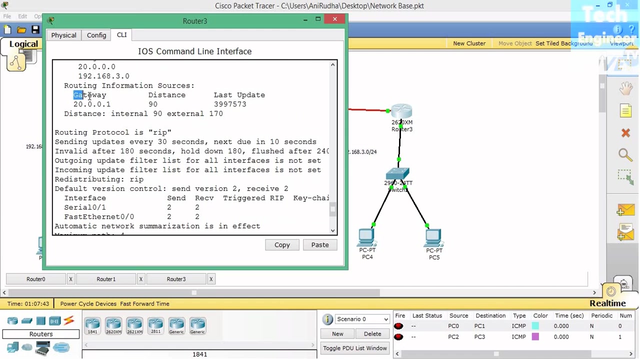 20, AS number is 20 with EIGRP and its internal routing is 90,, the distance is 90,, external is 170 and the RIP version having 120 the distances. So if you see the distance, for example here, routing information source. so, for example, 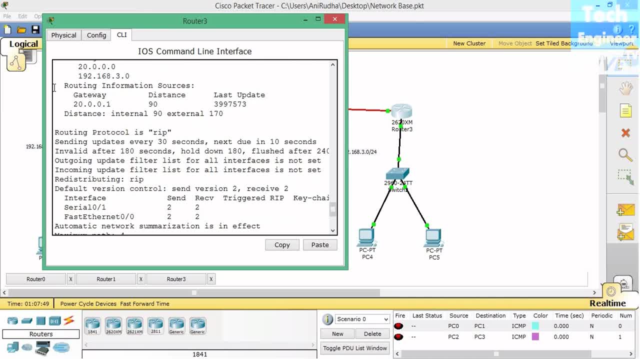 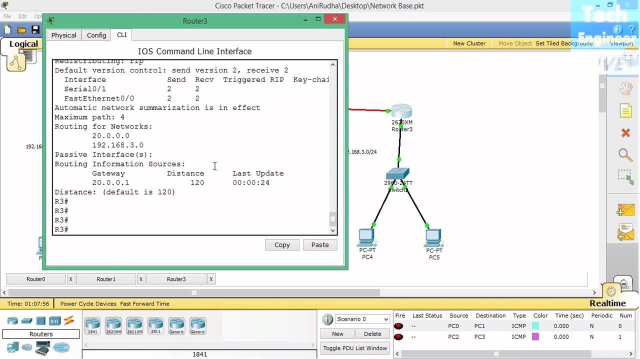 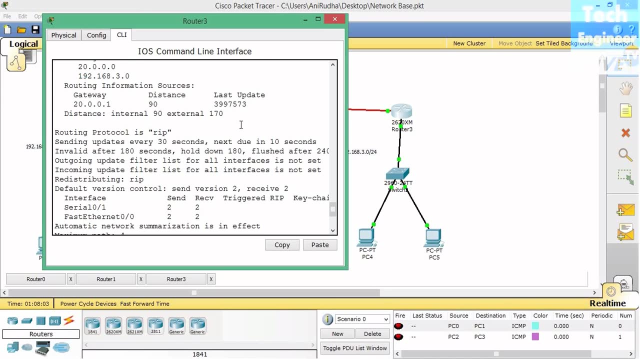 this is where we are talking about the routing information sources. so gateway is 20 is 1,, distance is 90, and here gateway is 20 is 1, distance is 120.. So the routing protocol and for that reason you can see the EIGRP, is 20, the distance 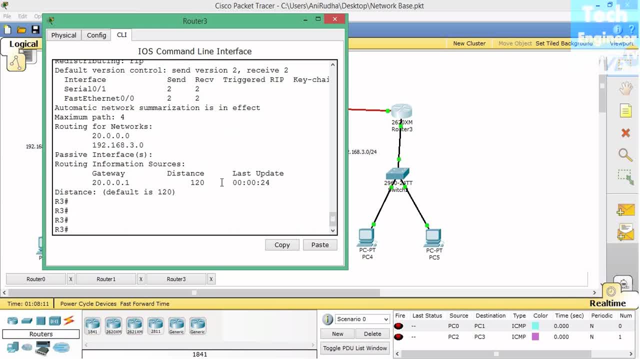 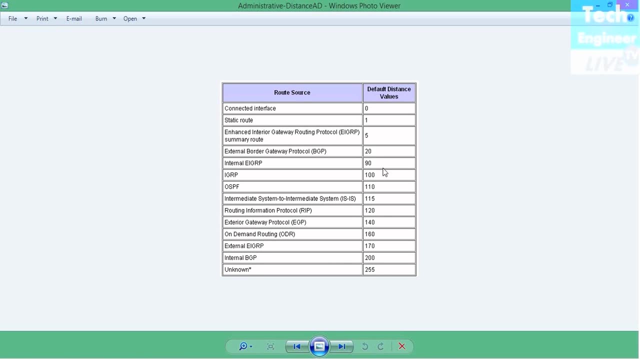 is a bit higher that, in that the distance value is 90 and RIP is 120.. So they have a chart, they have following protocols and they have the value and according to it, for example, if you put IGRP, if you enable IGRP, then it would be one step lesser. 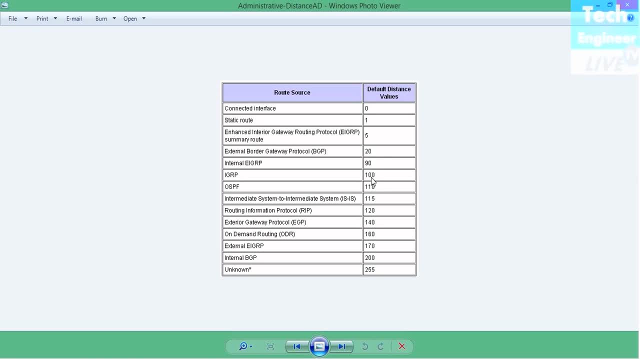 than EIGRP or higher than RIP. So it basically is all about the value evaluation of your believability in a route, the protocol, who's most trusted one and who's not. So whatever protocol you're using, just remember one thing: If you want to create a trusted network, make sure then go with the latest version of a protocol, whatever it is. For example, it's EIGRP in this case, So go with it. Or external BGP, But this is how the ADOI work.